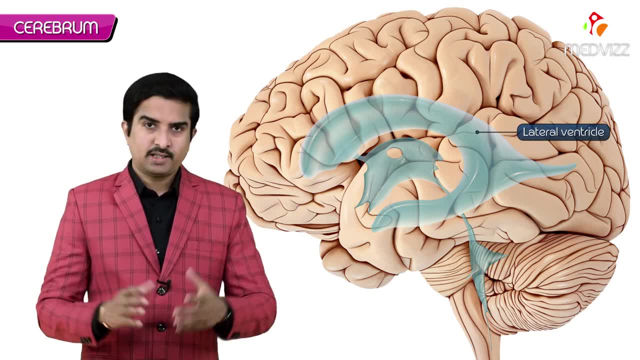 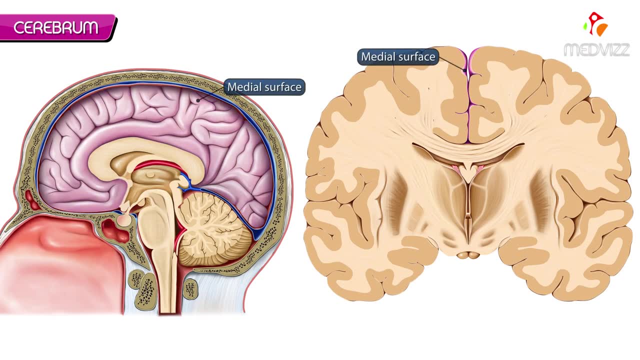 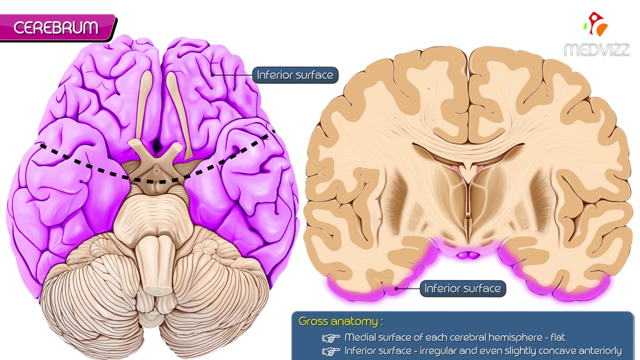 the cerebrospinal fluid. Now let us concentrate on the gross anatomy. If we see the medial surface of each of the cerebral hemispheres over here, the medial surface is flattened and inferior surface is extremely irregular and and even it is slightly concave. So the concavity is predominant more anteriorly when compared. 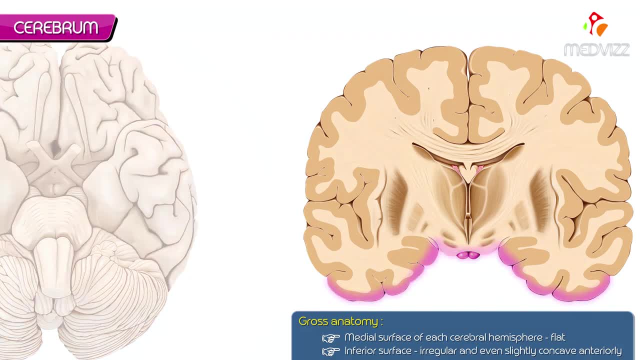 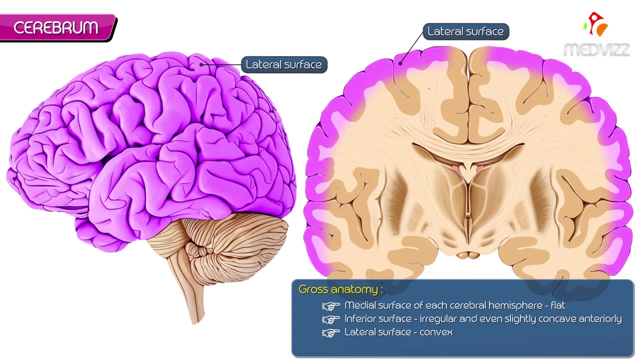 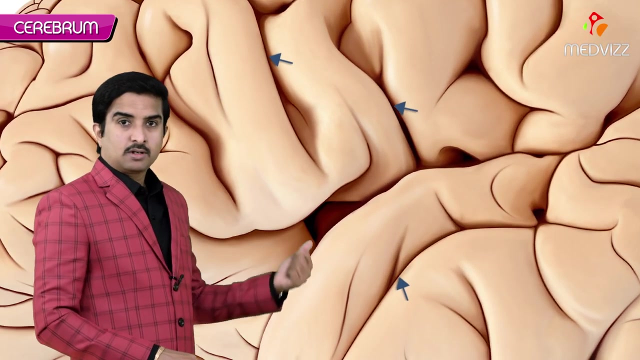 to that of the posterior aspect of the cerebrum, but while the lateral surface, where we can see here the lateral surface, is convex, So they are all lined by the cerebral cortex. So the surface of the cerebral hemisphere is divided by grooves called sulky and into 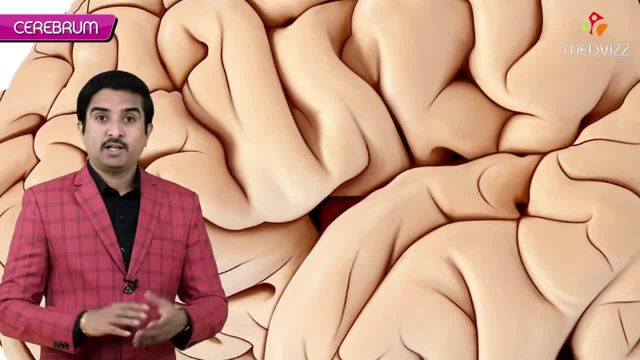 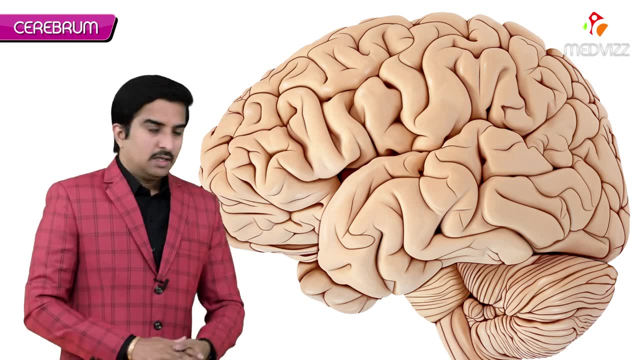 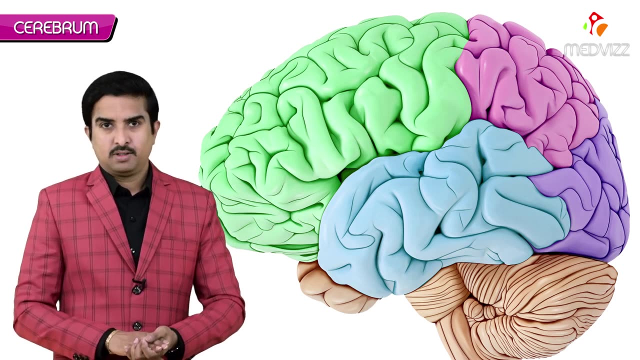 ridges called as gyric. Now let us talk about the division of the cerebral hemisphere according to the lobes. So each of the cerebral hemisphere is divided into 4 lobes of unequal size, Out of this frontal lobe, 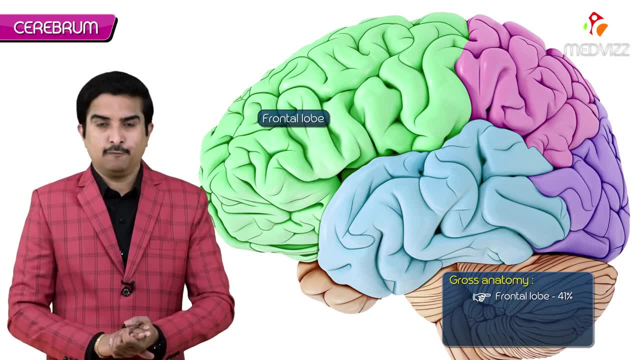 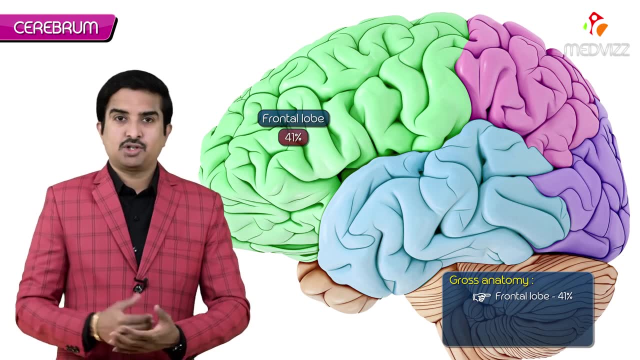 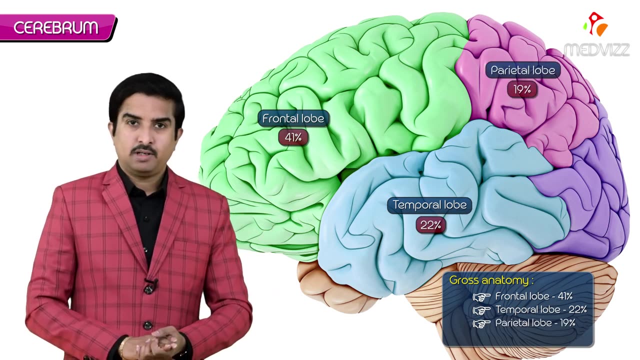 Which occupies the greater percent of the neocortical volume, which occupies approximately 41 percent of the total cerebrum. Second comes to the temporal lobe, which is 22 percent, the parietal lobe, which is 19 percent, and occipital lobe occupies 18 percent of the 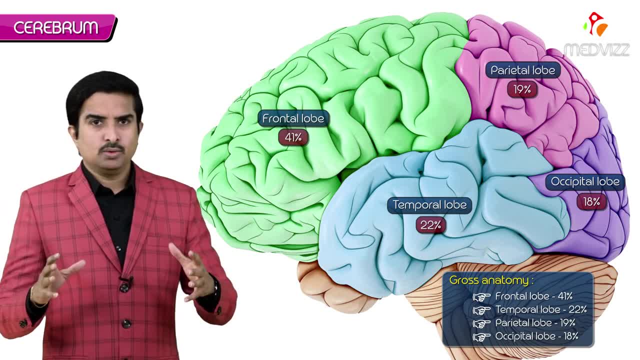 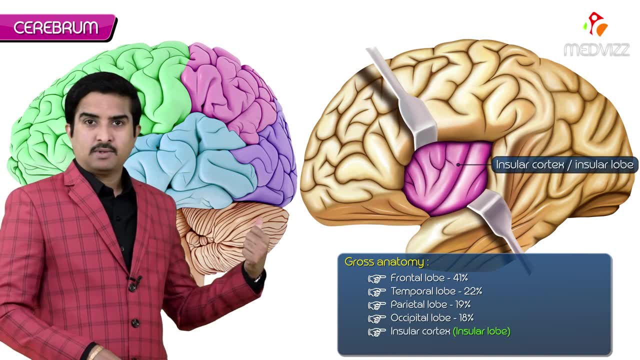 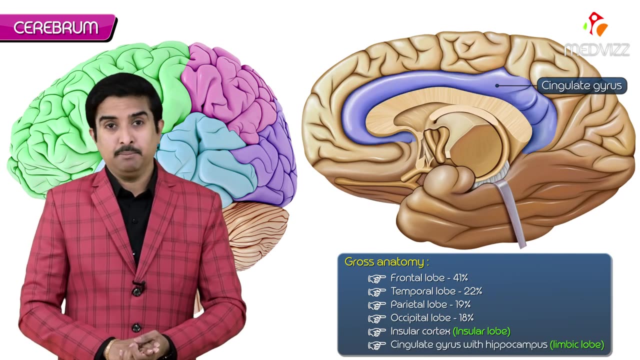 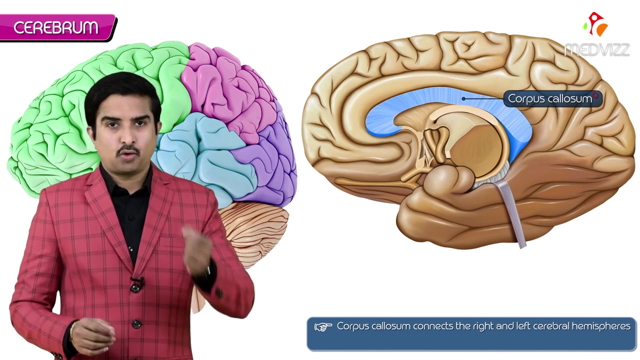 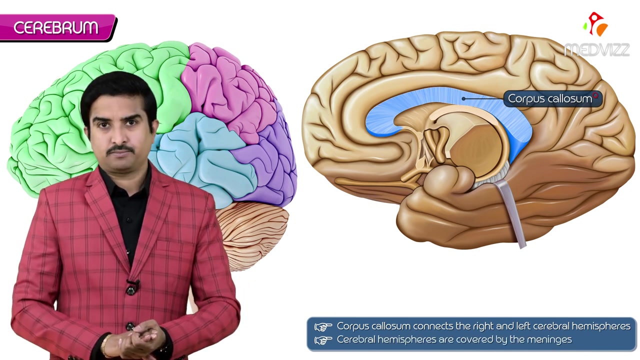 cerebral volume. In addition to these 4 lobes, some of the authors also refer to the galengine. Now, the macrophờ is an area which is very narrow and in the text about the sacral lobe, the villus is flowered out of a initial 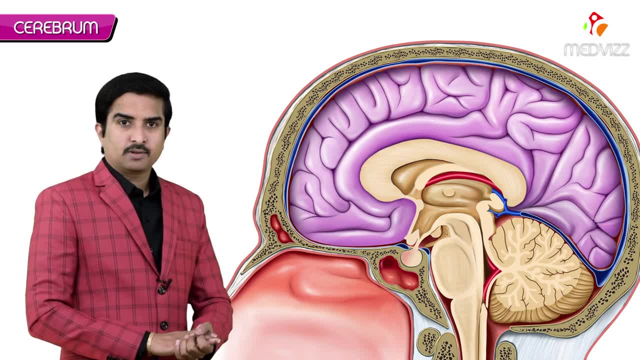 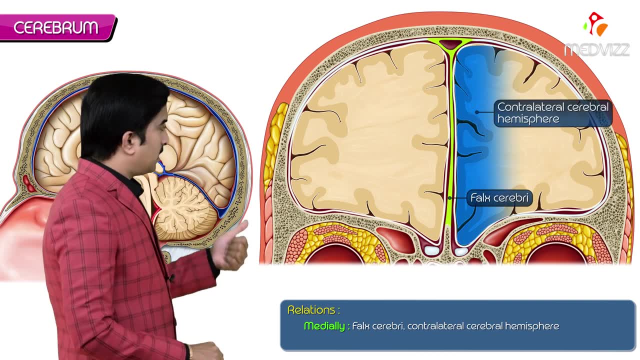 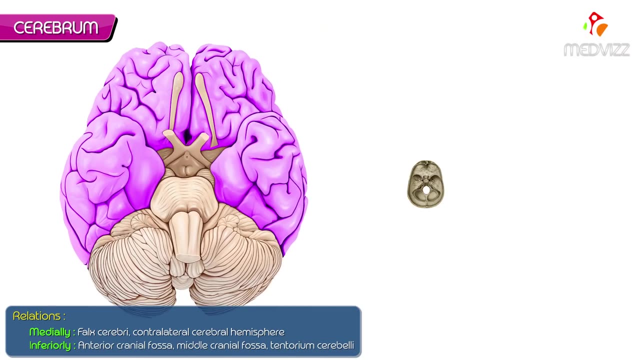 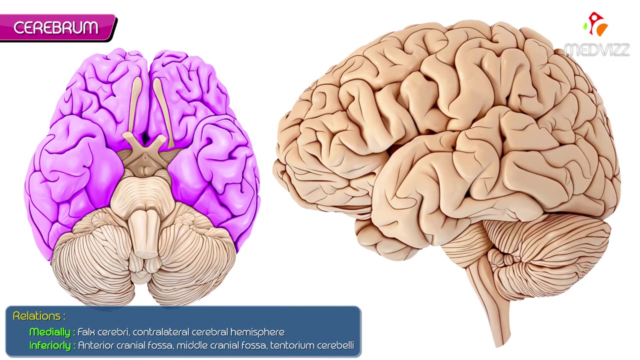 co guided. If we talk about the medial relations, first medially we have a structure called as fac cerebri and also we have the contralateral cerebral hemisphere but where, if we see inferiorly, we have the anterior cranial fossa, middle cranial fossa, as well as we have a tentorium. 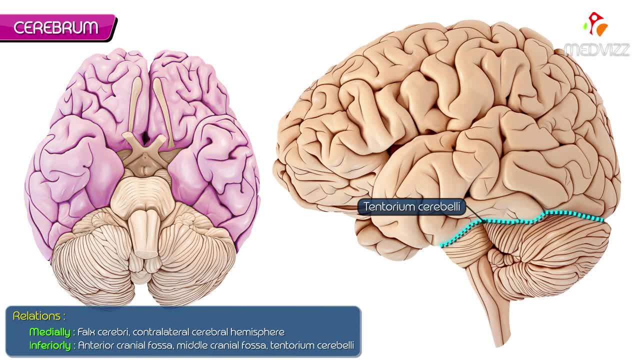 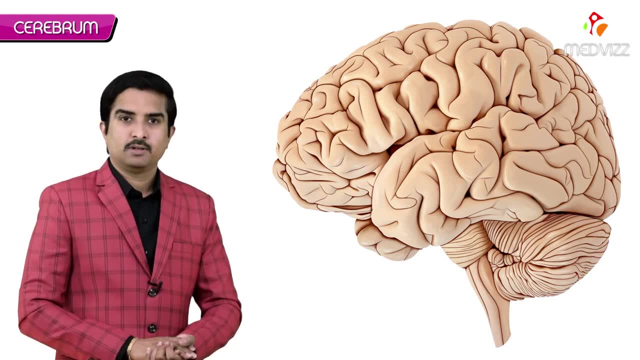 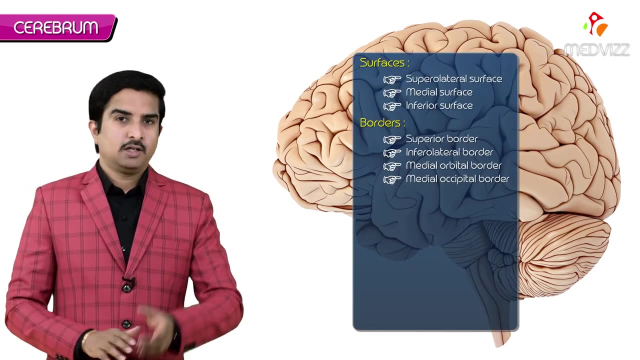 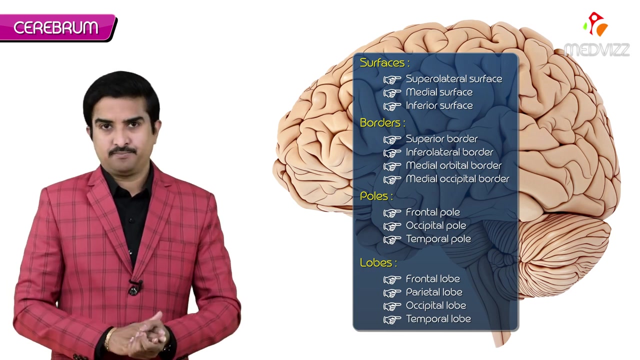 cerebelli, which is a tent like structure. Now let us talk about the external features of the cerebrum. Each of the cerebral hemisphere has three surfaces, four borders, three poles, and it is divided into four lobes. Now we have to discuss all these in detail. 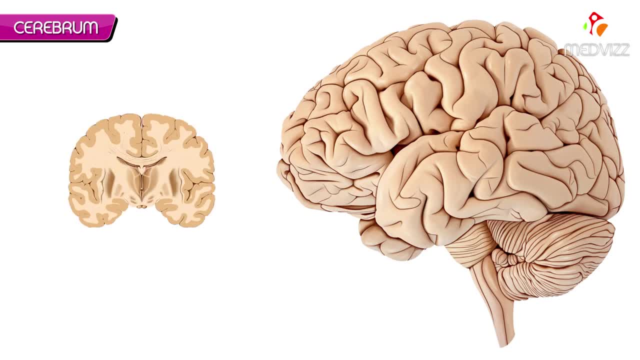 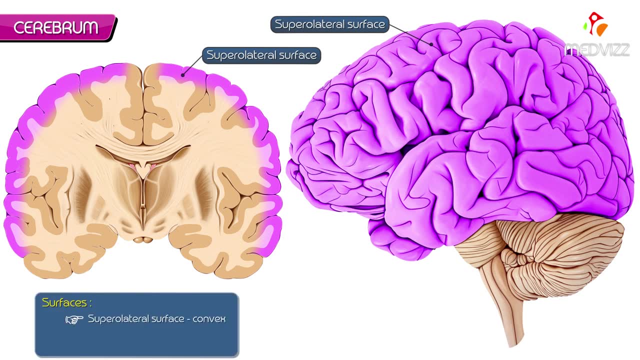 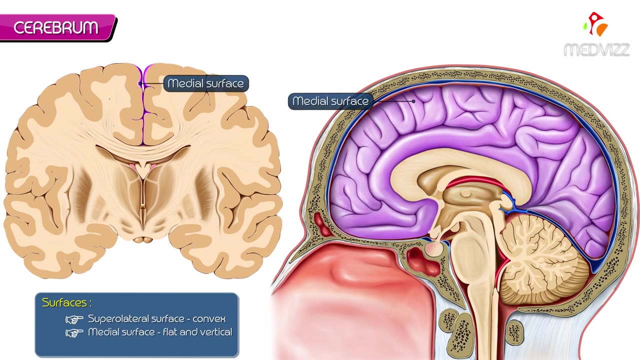 What are the three surfaces of the cerebrum? The first one is the cerebrum, The second one is the supralateral surface. So this supralateral surface, what we are seeing here, the supralateral surface, is convex in nature and whereas the medial surface, which is flat, and it is vertical completely, and 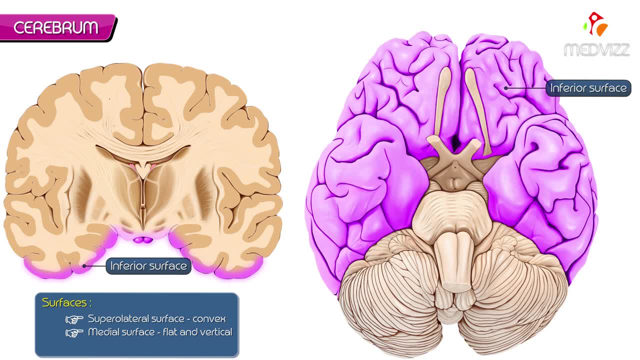 if you see the inferior surface here, the inferior surface is irregular and it is divided into an anterior part, which is called as orbital surface, and posterior part, which is called as the tentorial surface. So this is the anterior surface, So these are the surfaces of the cerebrum. 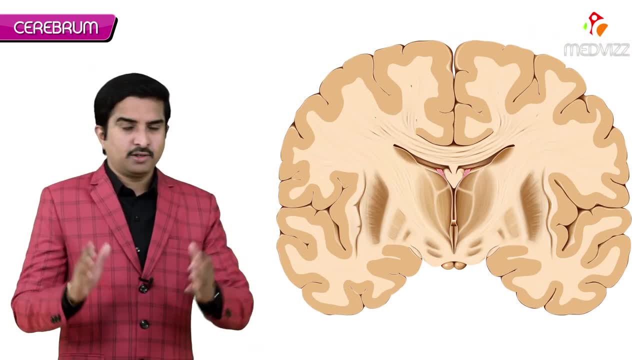 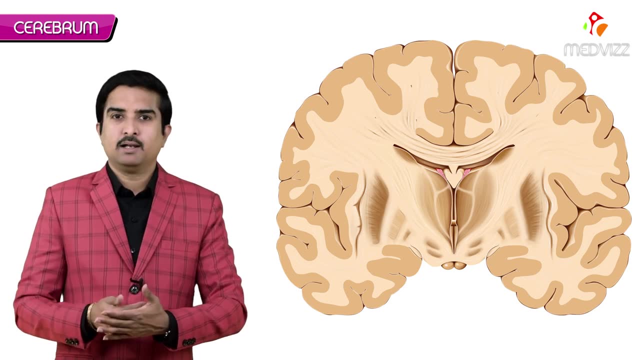 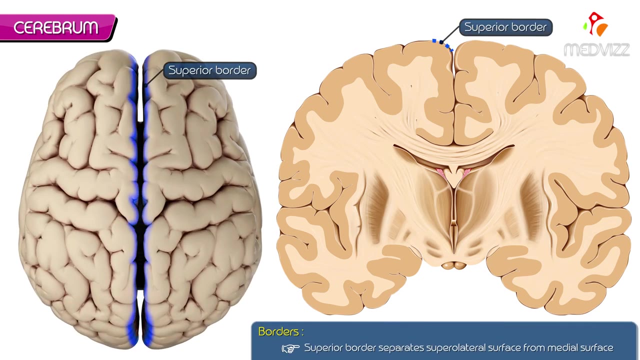 And next is about the borders. How many borders are present? There are totally four borders: superior infralateral, medial right, that is, medial orbital and medial occipital. So the superior border here separates the supralateral surface mainly from the medial. 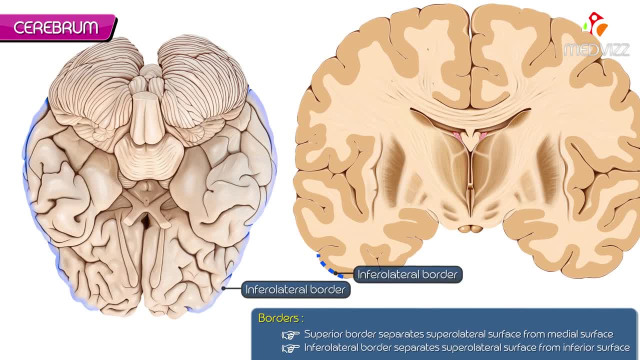 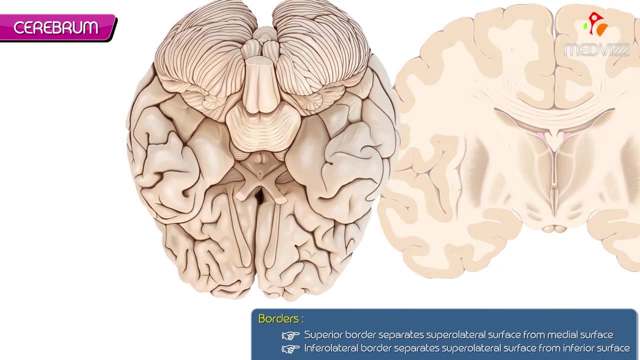 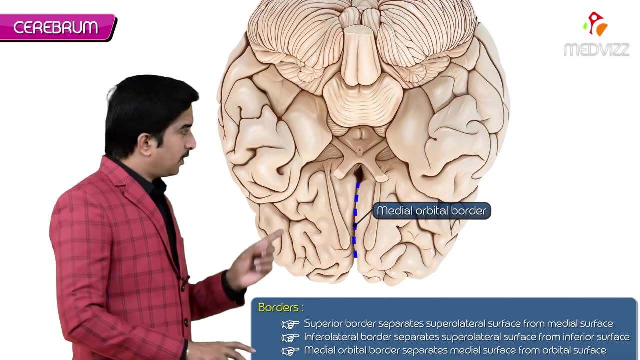 surface Whereas the inferior surface. So this is the superior surface. The infralateral border separates the supralateral surface from the inferior surface. When we talk about the medial border, that is, the medial orbital border separates the medial surface from the orbital surface. 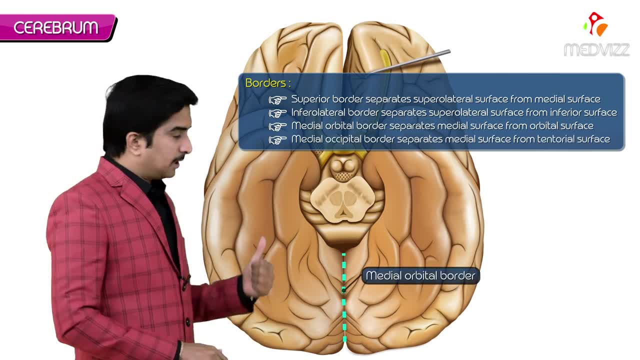 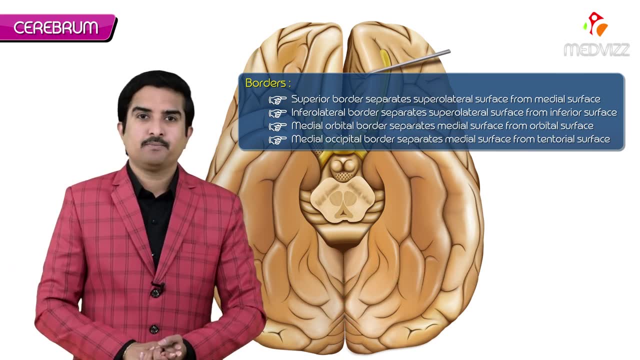 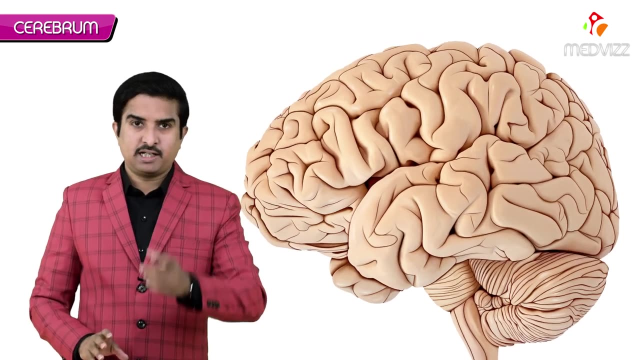 In the same way, the medial occipital border separates the medial surface with the tentorial surface. So these are the borders of the cerebrum. Next is about poles. So when we talk about poles- first one, let me talk about the frontal pole-